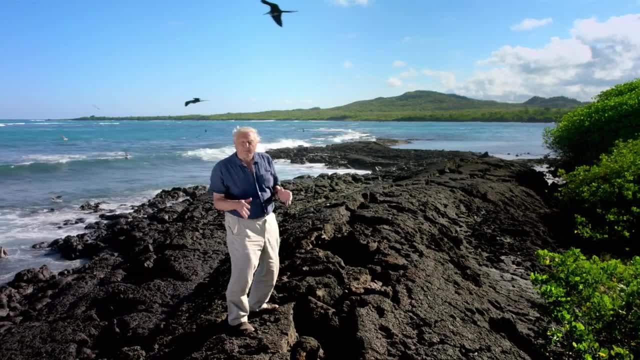 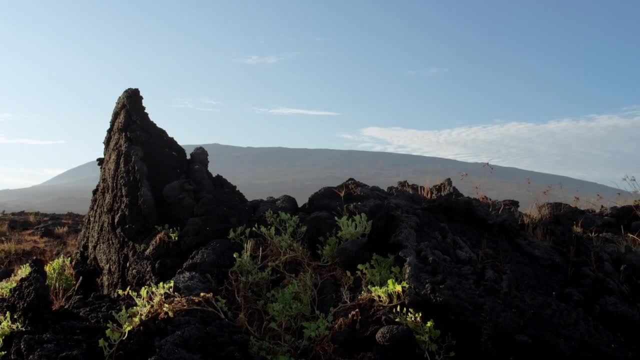 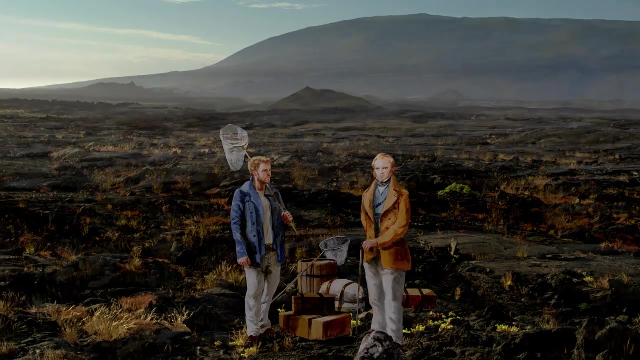 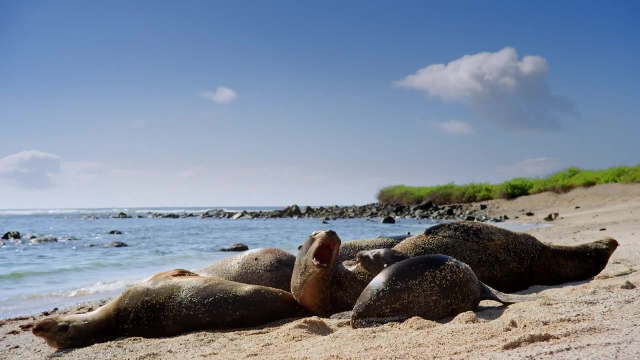 And the 26-year-old Charles Darwin stepped ashore to explore. At the time, very little was known about the natural history of the islands. Darwin initially was fascinated by its geology, But it was the animals that gave him his historic insight. 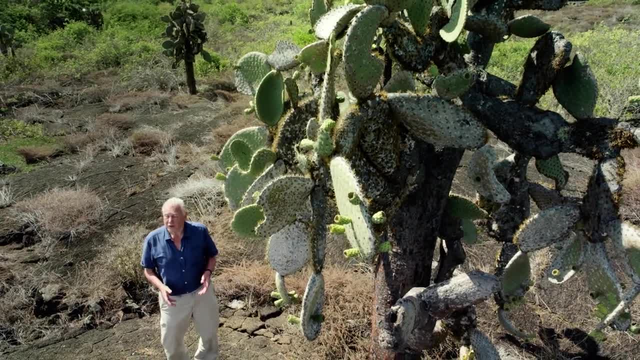 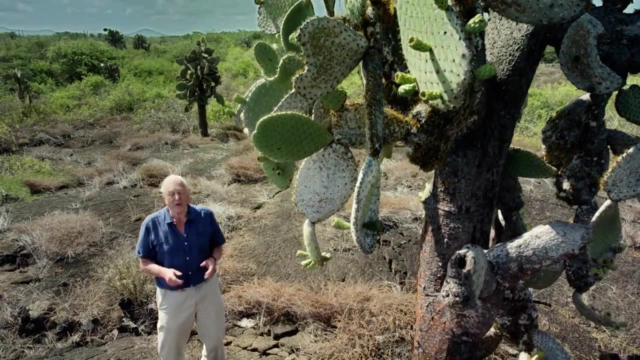 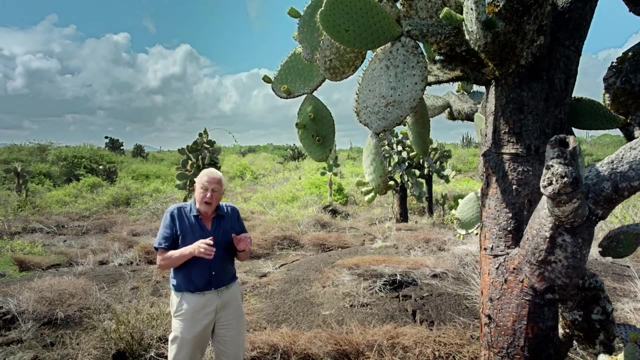 Darwin was only on these islands for five weeks, But in that short time there were things he saw and conversations he had which stuck in his mind. For example, the British vice-governor of Floriana Island said that he could tell which island a giant tortoise came from simply by the shape of its shell. 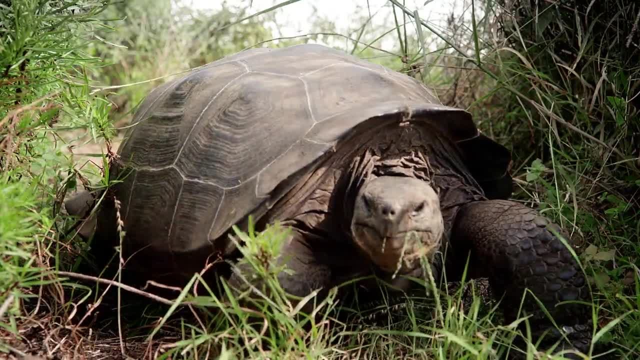 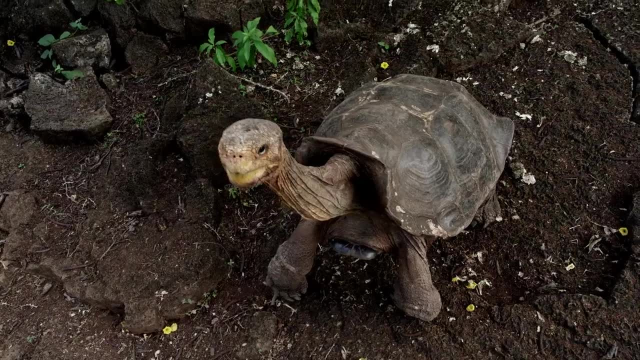 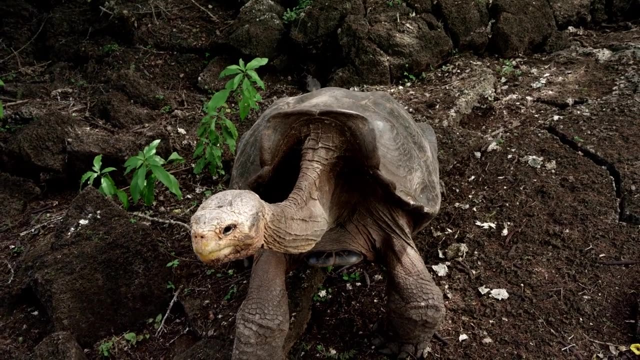 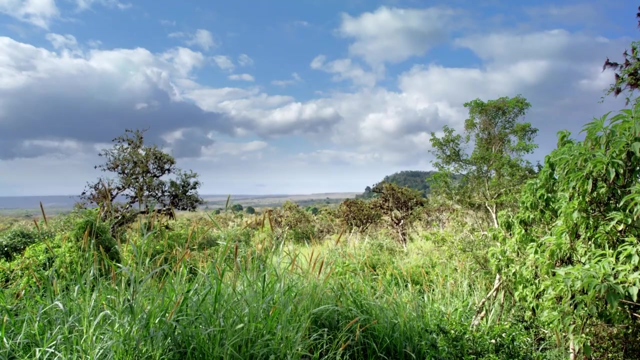 He pondered on the vice-governor's casualty And he made a remarkable remark: Why were populations of tortoises on separate islands all slightly different from one another? He set about making a collection of animals and plants from all the islands he visited. 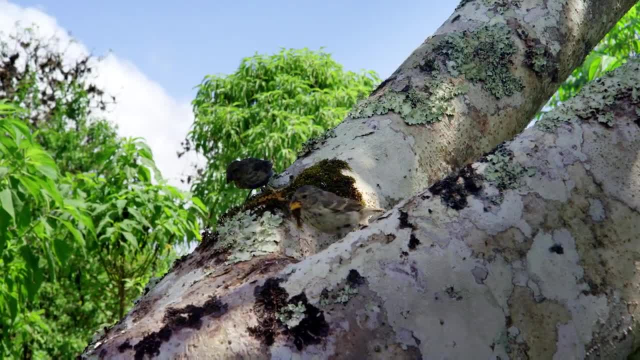 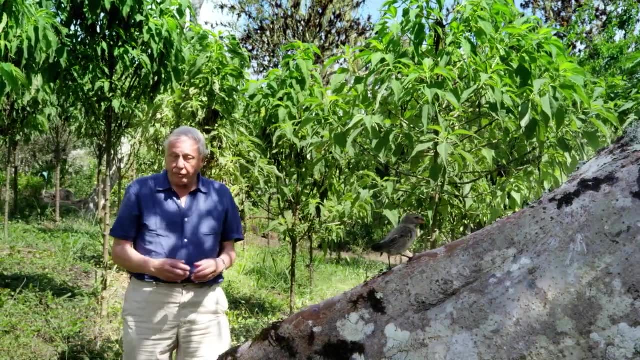 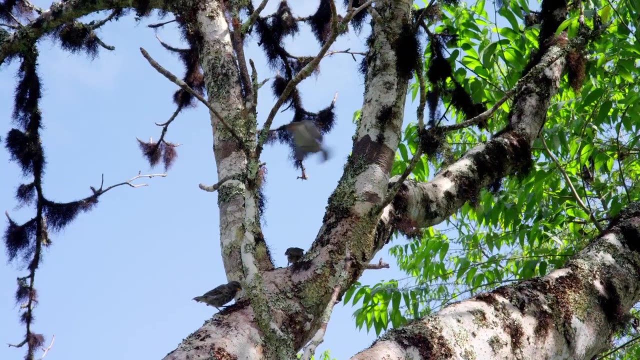 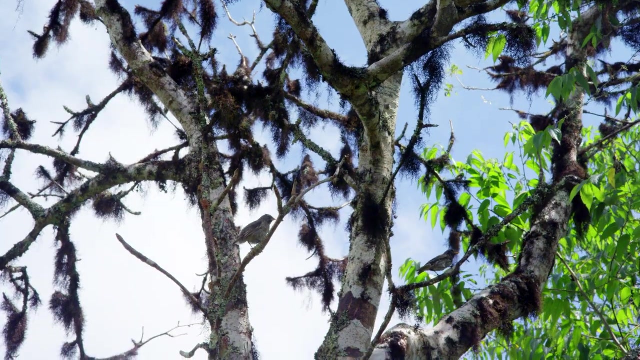 Although it was the tortoises that first alerted Darwin to the differences between animals on different islands, it was his collection of these undramatic little birds, the finches, which provided him with the most substantial evidence for his great theory. We now know that the ancestral Galapagos finches arrived in these islands. 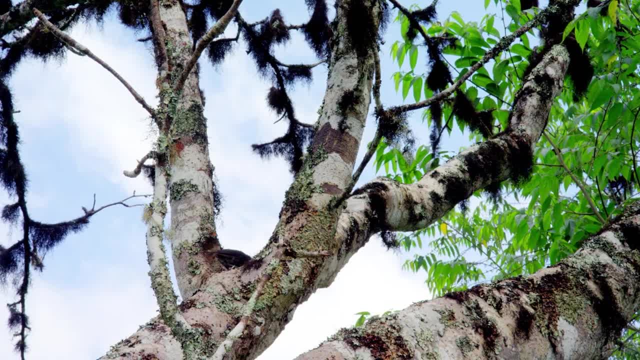 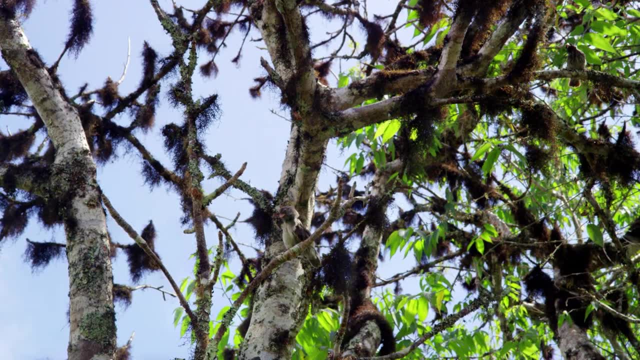 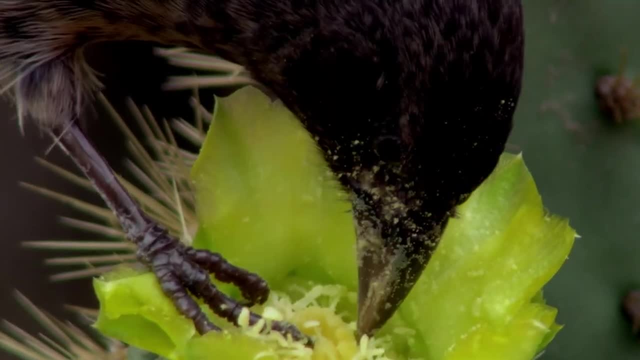 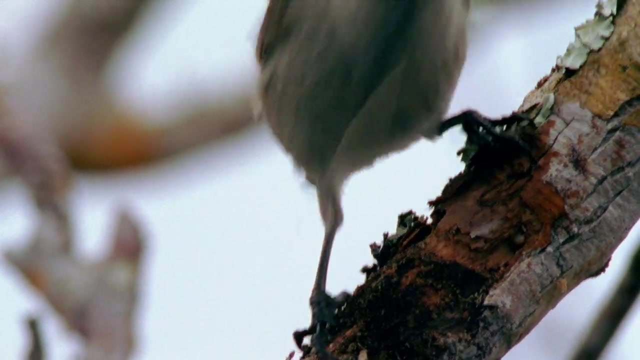 about two million years ago. Since then, they have diversified into a number of different species. Today there are 13 of them distributed throughout the archipelago. Each has its own special talents. The woodpecker finch has discovered how to use a tool to winkle grubs out of their burrows in the branches of trees. 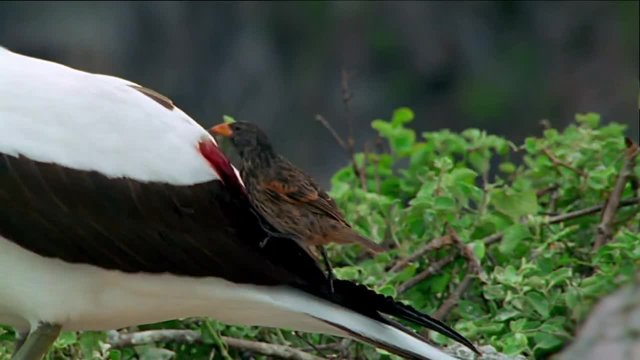 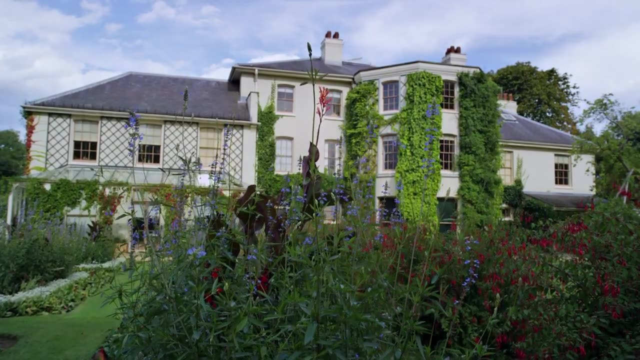 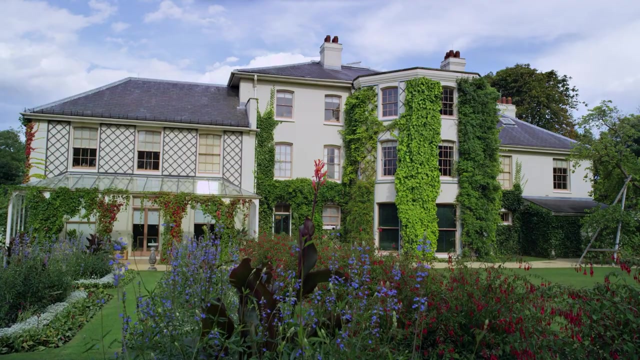 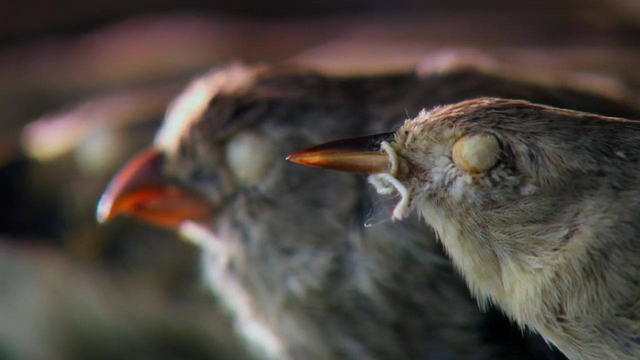 The vampire finch has learned how to extract blood from sitting birds. Darwin, when he returned to England, brought back with him a wide variety of specimens of all kinds, And he spent years studying his collections. He had a range of finches from several of the islands. 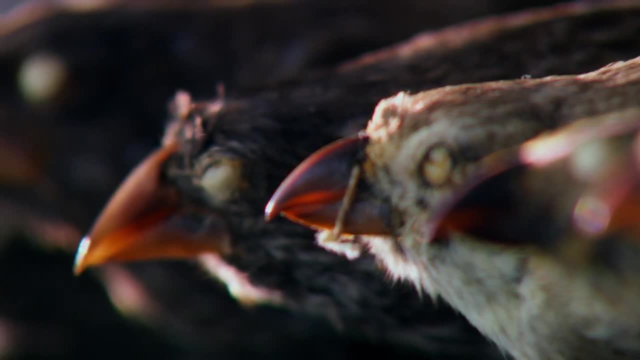 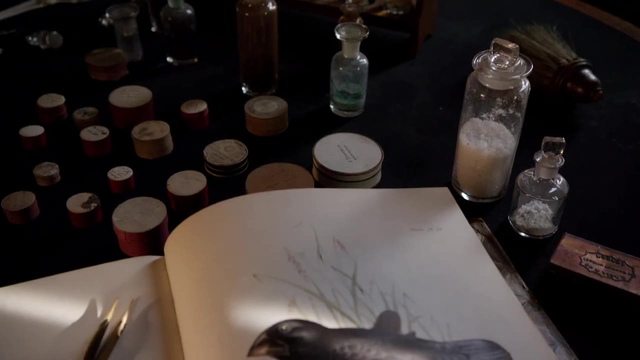 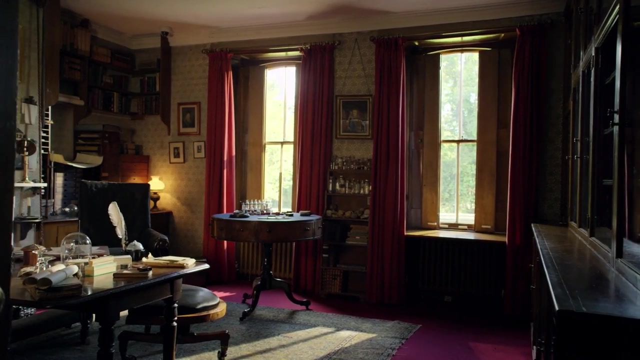 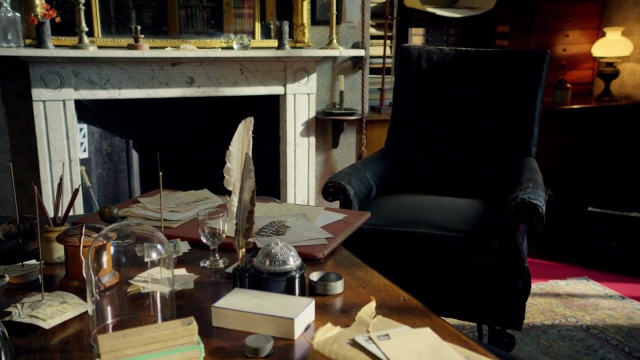 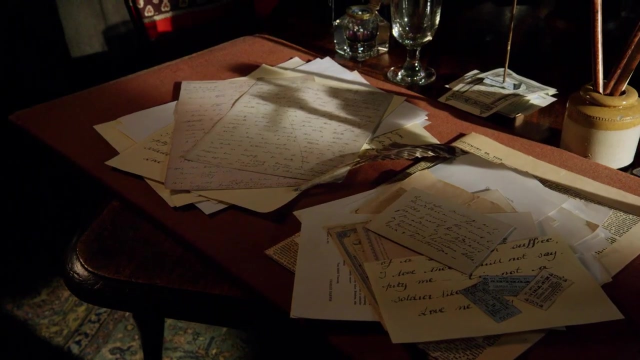 and he noticed one particular way in which they differed: They had beaks of different sizes. Why, An idea grew in his mind: It would also apply to tortoises, maybe to all animals and plants wherever they occurred. Painstakingly meticulously, he started to accumulate evidence from all over the world to support his idea. 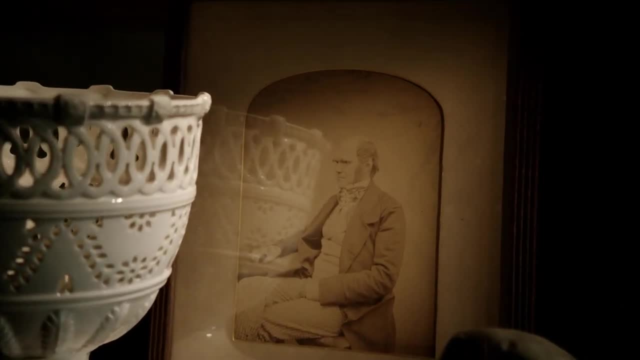 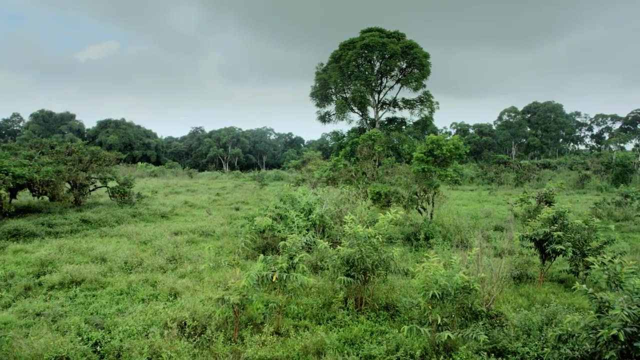 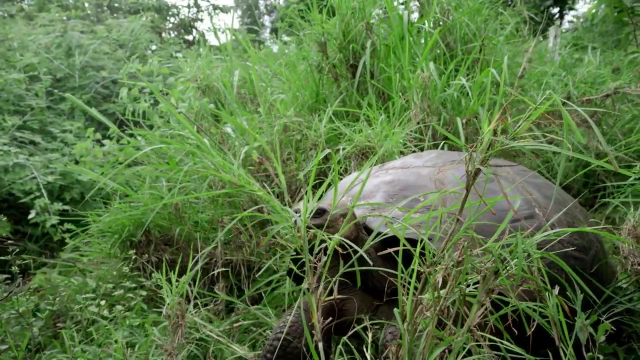 And he called the process that produced new species evolution by natural selection. And nowhere is its workings more vividly evident than here, where it first occurred to him, in the Galapagos. He realized why it was that there were several species of giant tortoises. 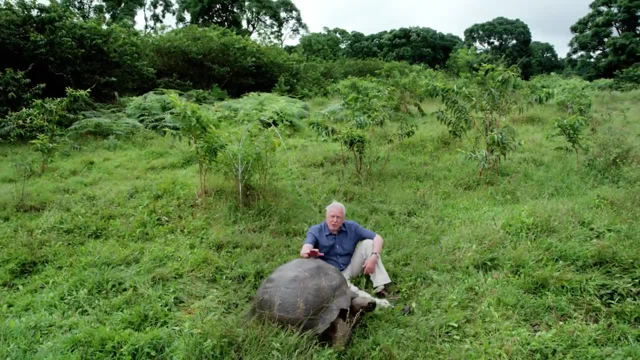 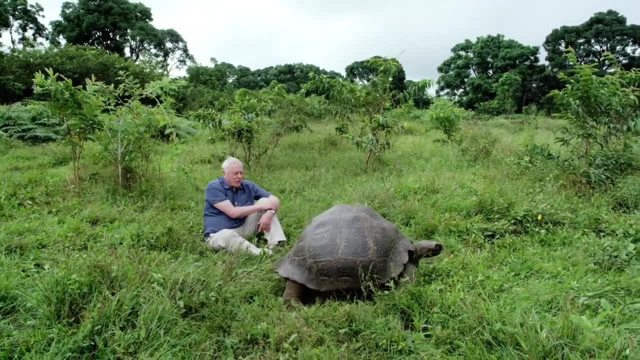 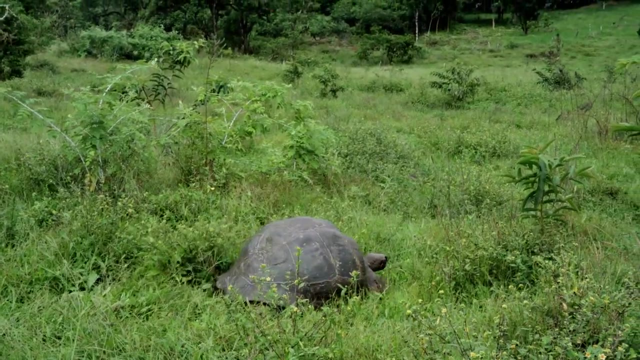 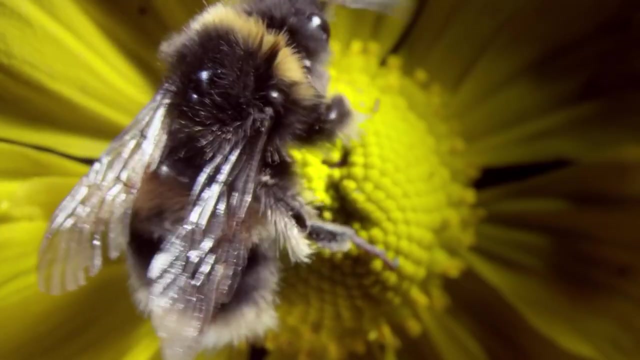 That original species probably had a high domed shell like this one, And that's very useful on well-watered islands like this, where you have to barge your way through the vegetation. But on other islands there are other problems. Each and every species of flowering plant has its own unique evolutionary story that's closely coupled with the animals that pollinate it. But one family of flowering plant has developed this relationship in more complex ways than any other And in doing so has become the most numerous and diverse on the planet. There are an estimated 25,000 species of orchid. This family had a particular fascination for Charles Darwin, as he reveals in one of his letters that's kept here at Kew. 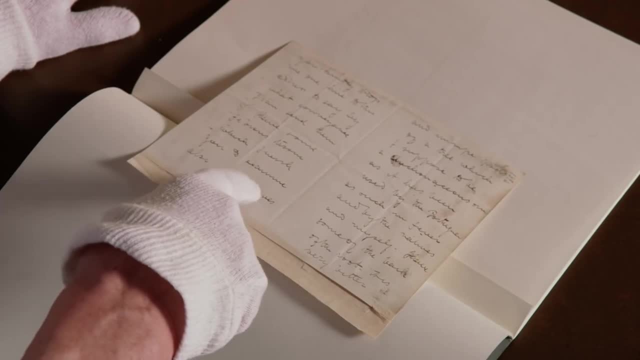 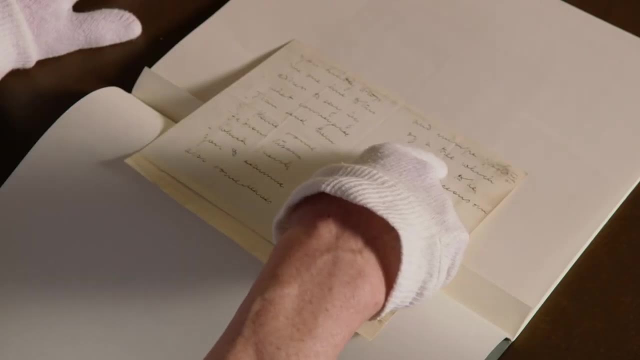 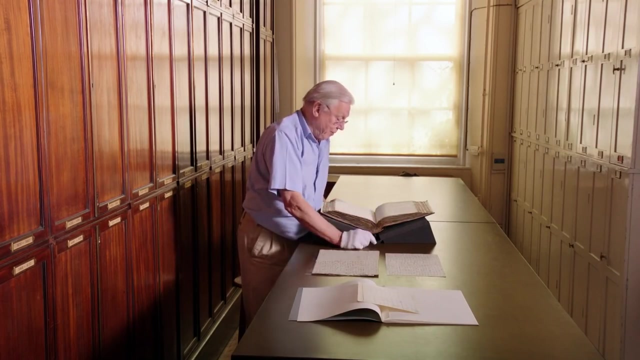 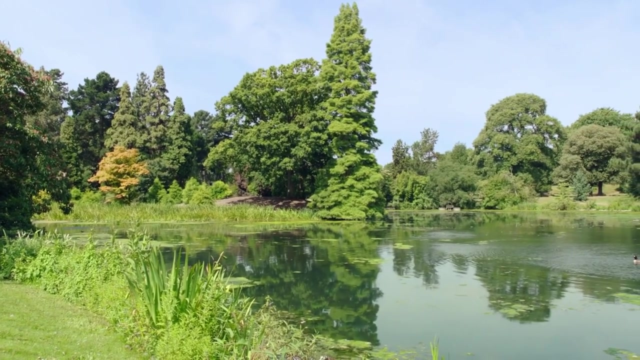 He says I have been extremely much interested with catecedum And indeed with many exotic orchids. Orchids have interested me as much as almost anything in my life, Charles Darwin. One species of these amazing plants can be found growing outside in the grounds of Kew. 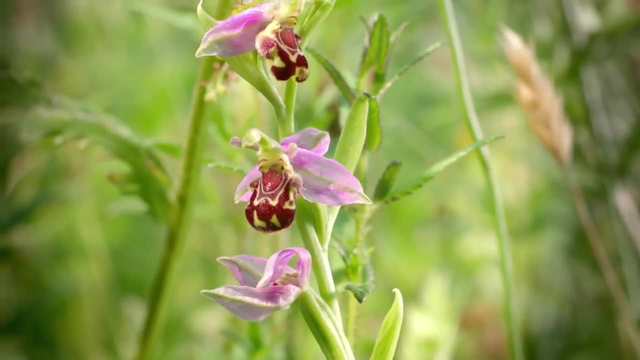 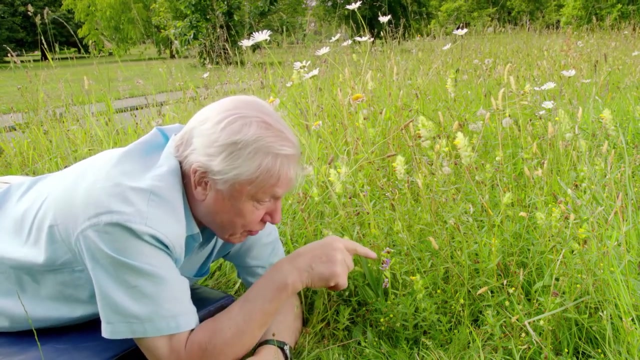 Orchids are extraordinary plants From many points of view, But one of them is that the lower lip of the flower is controlled by a special set of genes, So that means that it can evolve and change its shape and colour, while the rest of its petals remain the same. 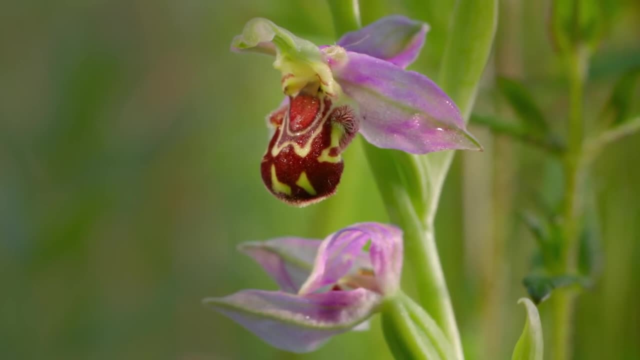 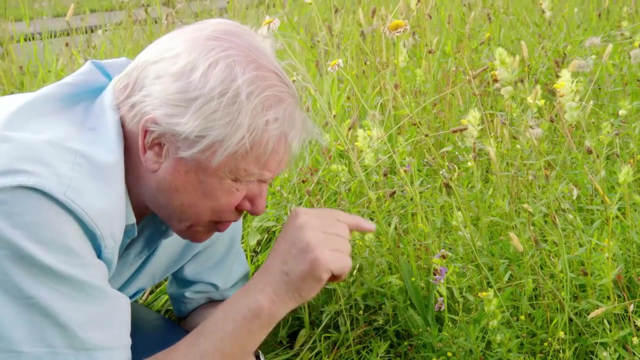 The lower lip of this little orchid has evolved to look roughly like a bee And people used to think that was a kind of warning To warn cows not to eke it, On the grounds that they wouldn't want to get stung on the tongue.